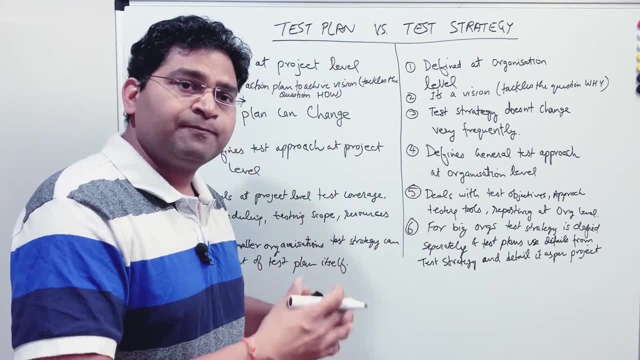 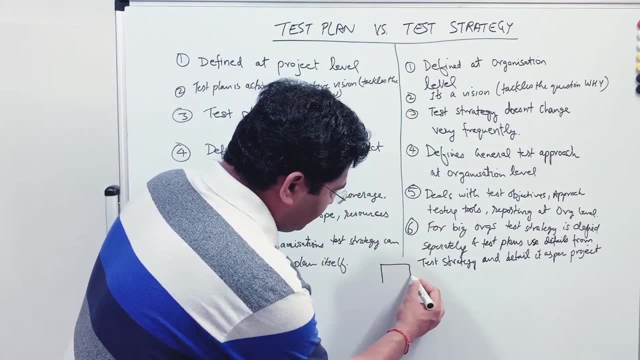 I'll call it test plan Here. I'll letter the point's. So, for example, if we are speaking about a tool like my account, It is mostly defined at the organization level. What this means is this: is the document, or test strategy is the document which is defined at the organization. 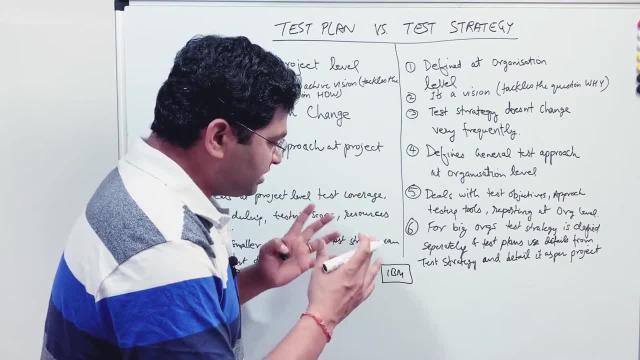 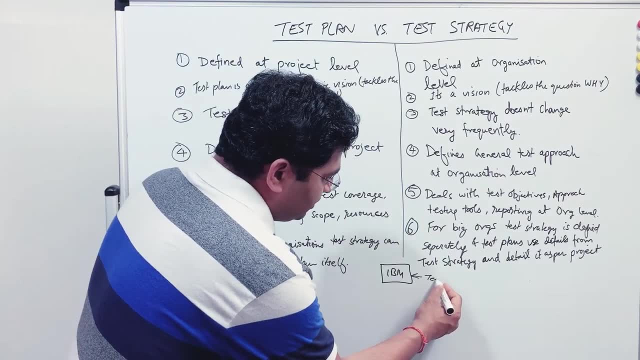 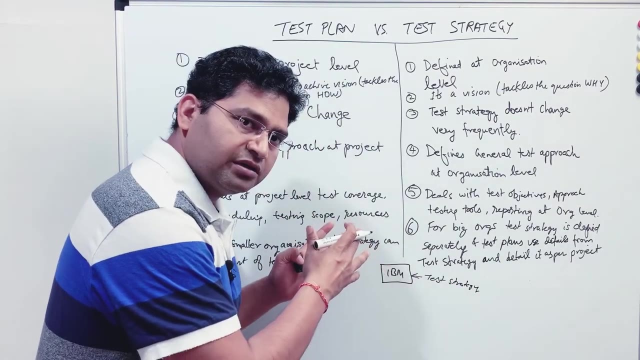 level. So, for example, hypothetically I'll take an example- I'll take an organization, say, for example, I'll take IBM, IBM, Al, intermittent, RM, E, K, 이, the org level. okay, now there won't be just one strategy for the whole organization as such. 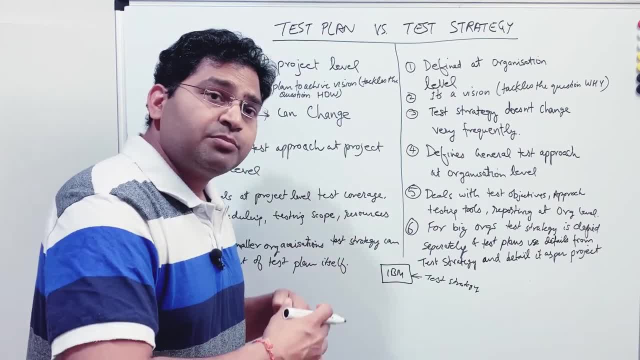 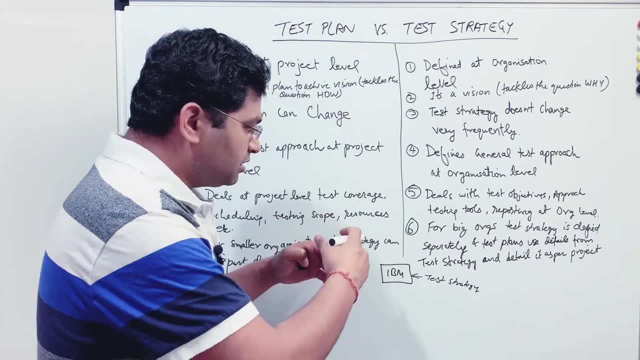 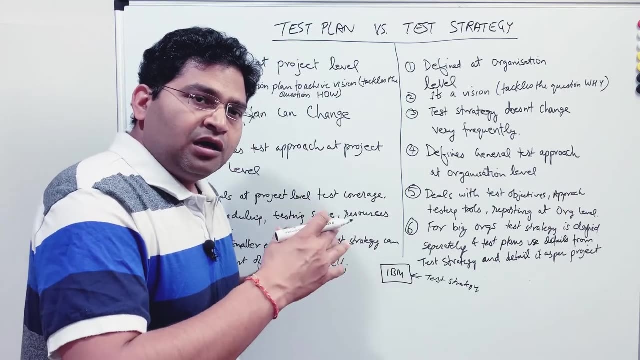 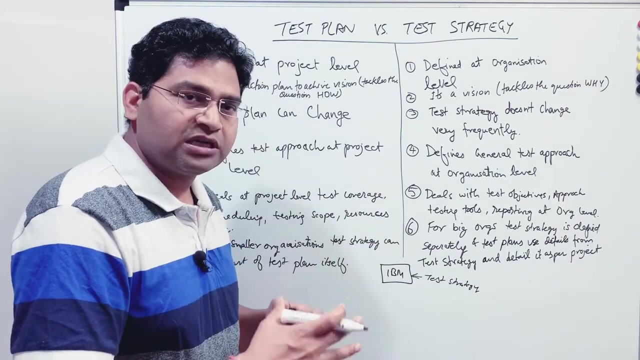 because ibm is a huge organization, right? so there can be multiple verticals within organization. there will be software vertical, there will be services vertical. so depending on the, the number of people or the number of projects within that organization, if they are sort of related, then that vertical can have one strategy or one test strategy and what usually goes into the test. 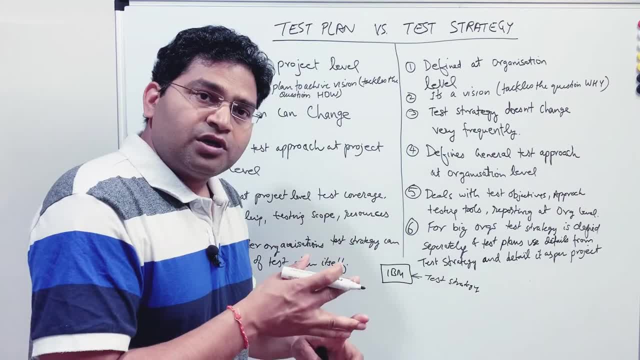 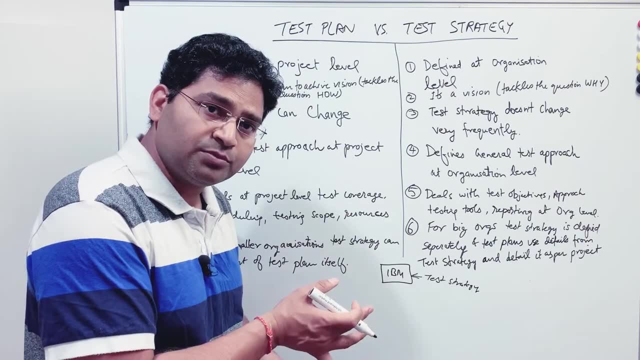 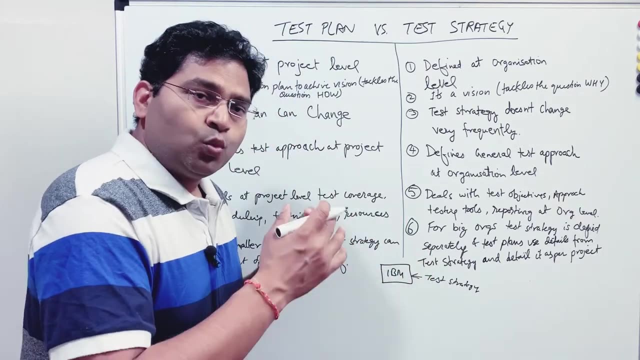 strategy document is: what sort of testing, how the testing will be approached, what tools will be used, what test management tools will be used, how the defects will be tracked. so all those general details of testing go into the test strategy document which, in turn, which in turn say for: 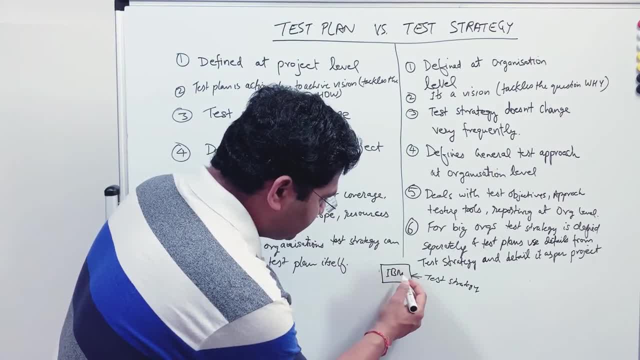 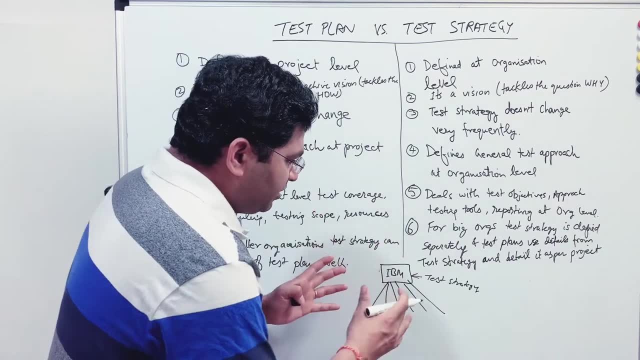 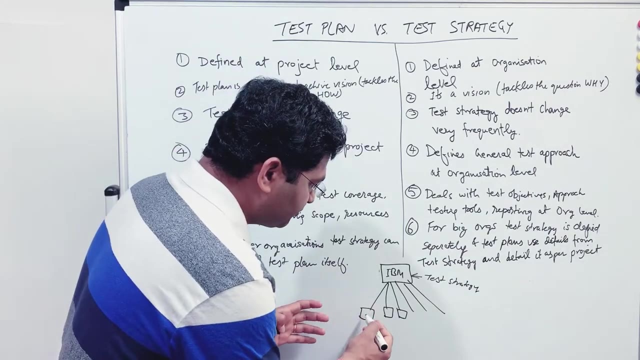 example, there is a vertical. so in you, in this organization- so i'll say ibm- there will be multiple n number of projects, right, so there will be multiple projects, and when these projects will start testing, or these projects will approach testing, what they'll do is they'll refer to the test strategy that is at the org level and they'll 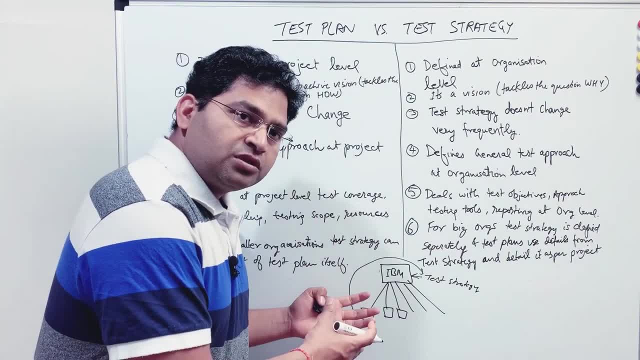 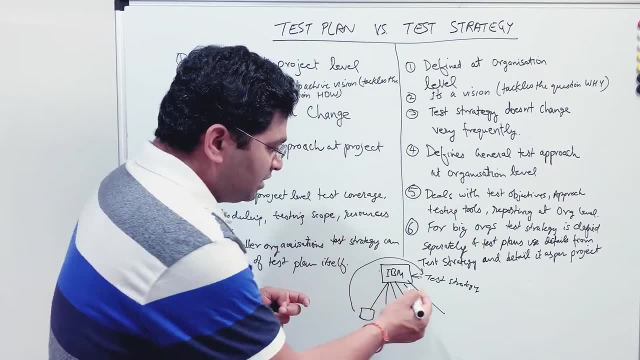 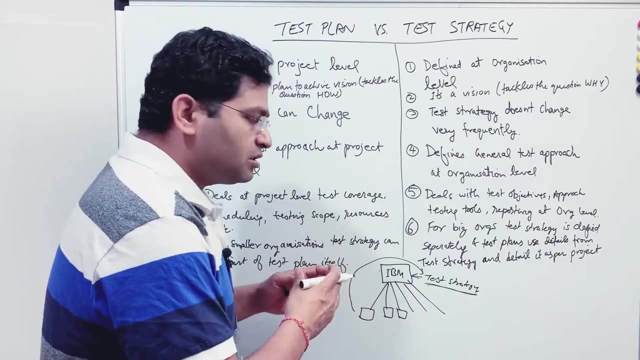 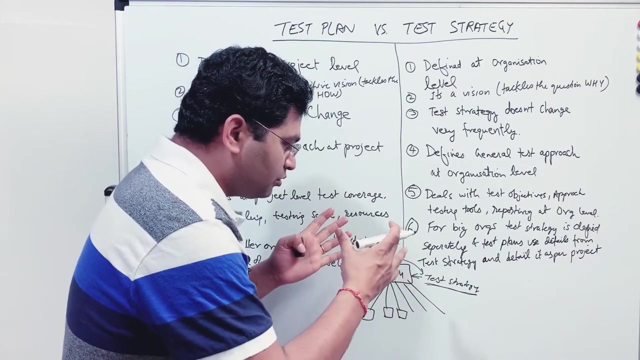 refer what all test management tools they can use, how the defects should be tracked, what all test artifacts need to be produced, etc. right, so this test strategy is important to make a common understanding, or define a common understanding across the organization so that any project that is being, you know, introduced within that. 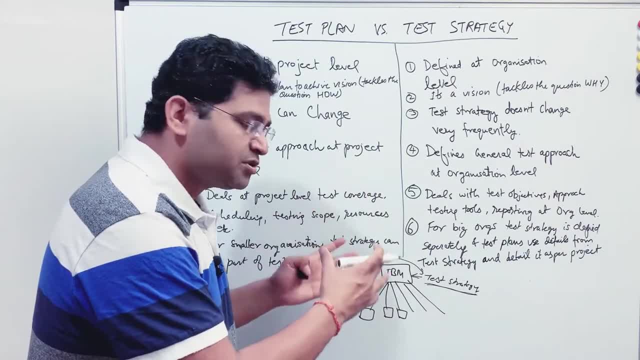 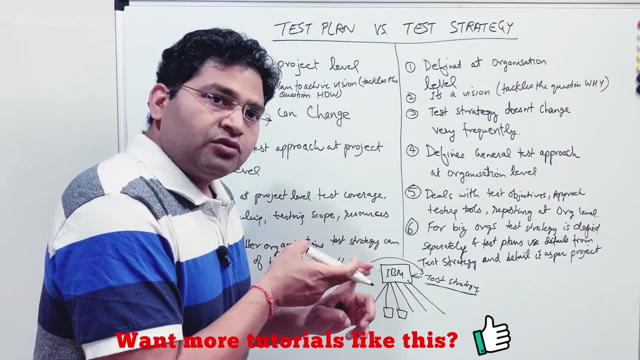 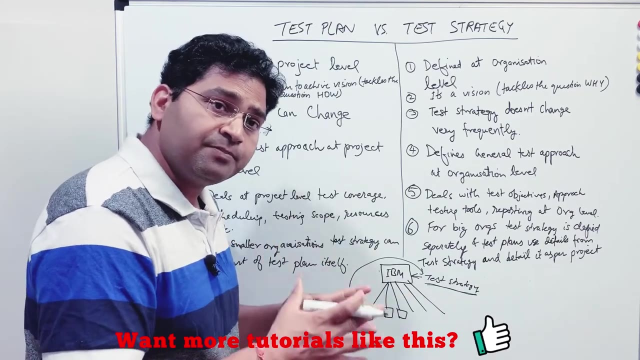 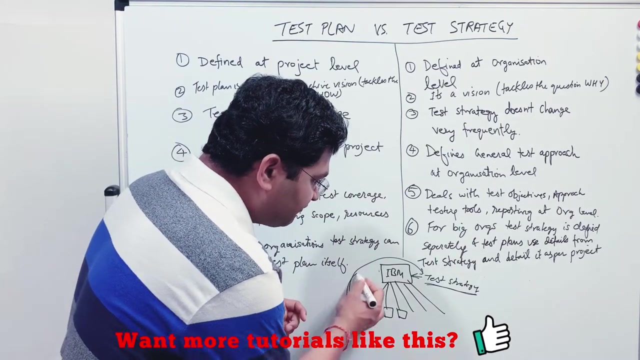 particular vertical organization follows the same strategy, follows or uses the same set of tools that are defined in the strategy and follows, you know, similar practices around the testing and the defect management. now there will be some modification within the test plan, so test plan will be at the project level and test plan will refer to this test strategy, right? so when the test plan 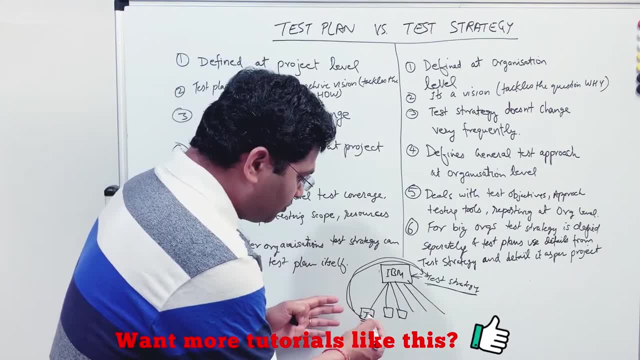 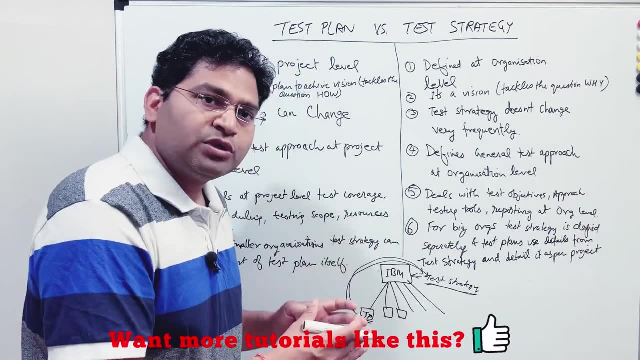 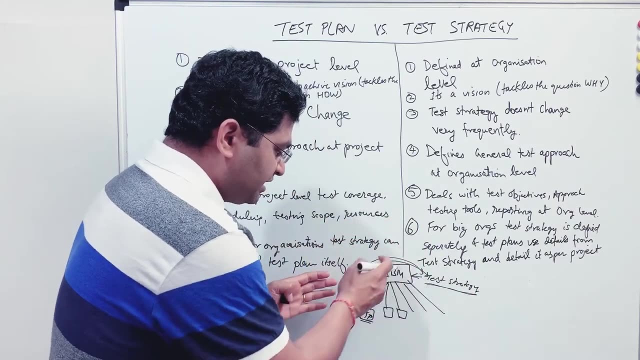 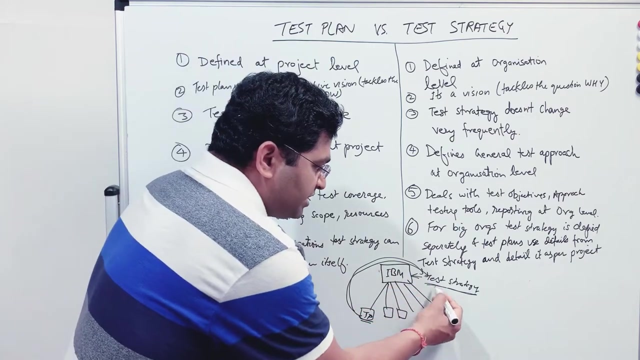 is written. it is very specific to the project. now, within this test plan, you will have the details about the project and how you will approach testing within the project. but you will take the key information from the strategy document- test strategy document- and then elaborate all those details within the test plan as per the project. right, because your test strategy will define you. 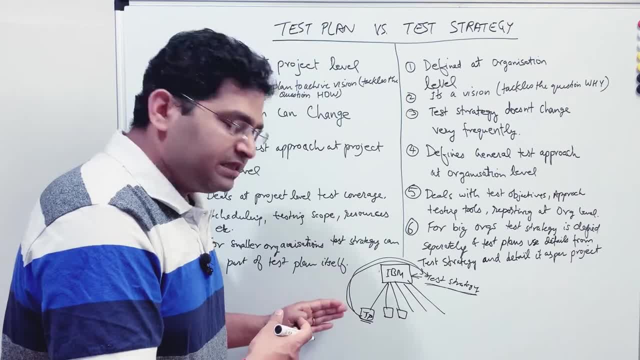 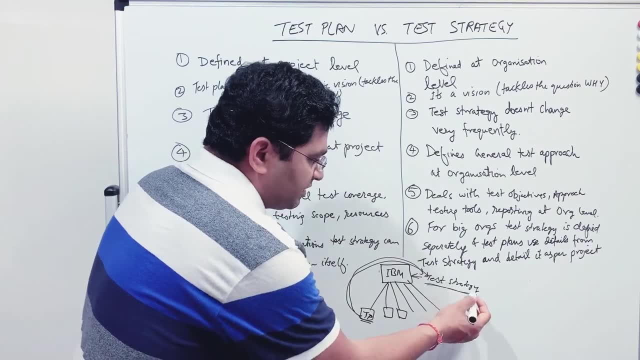 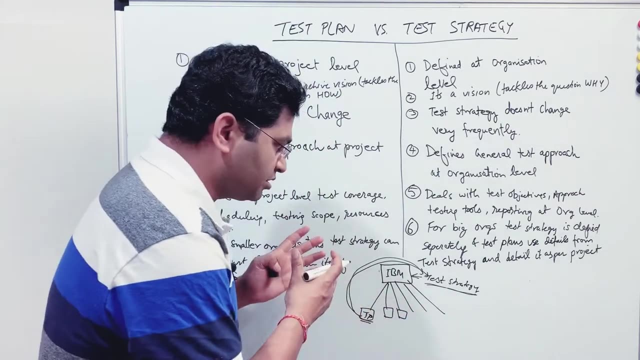 need to use this tool. this is the defect management process. these are the artifacts that you should usually produce. okay, so all that common information is defined at the test strategy level. why this is helpful is basically now. when you have this common understanding across the project, you will see that the strategy will be different for each individual and it will be a really 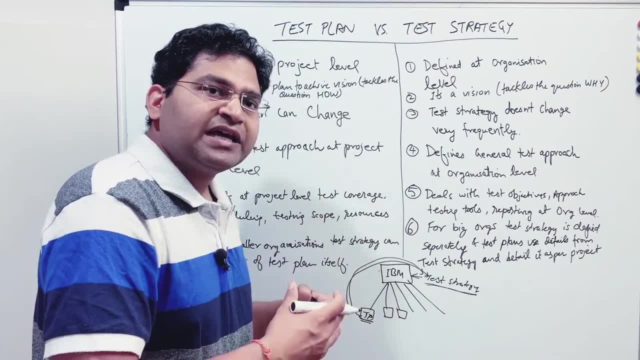 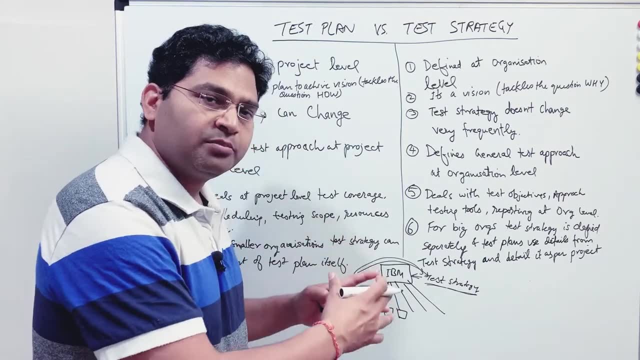 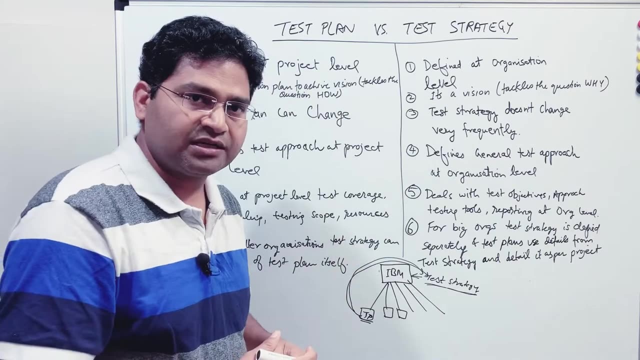 unique strategy for each individual in the process and how to apply that strategy in any type of project that you are interested in. also, the number of projects will vary. these projects will mostly use similar set of tools, similar processes, and this will reduce the complexities of managing multiple. 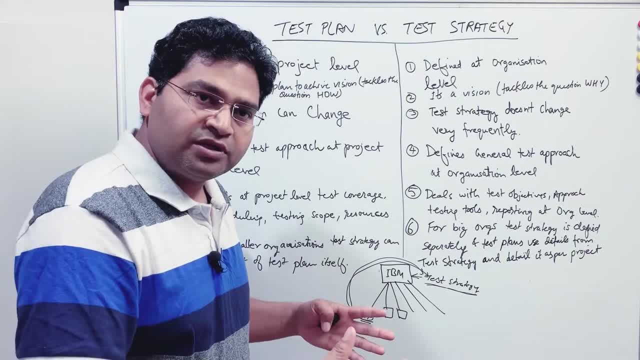 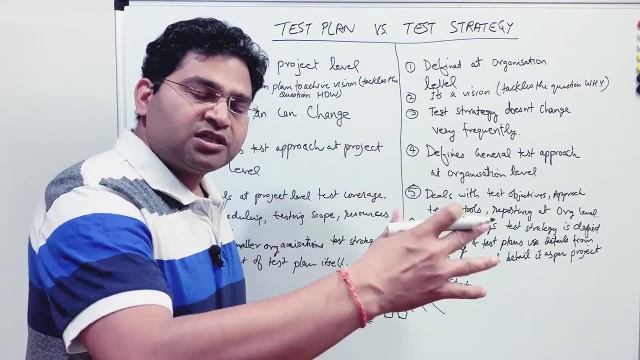 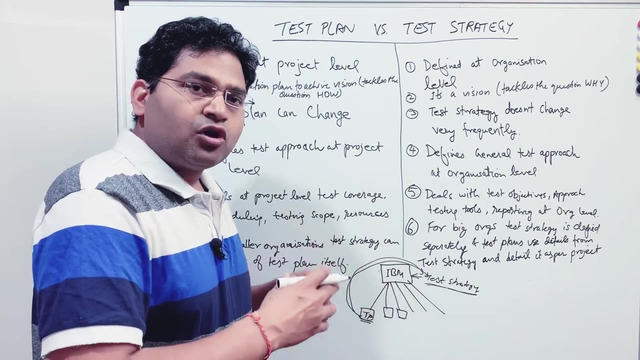 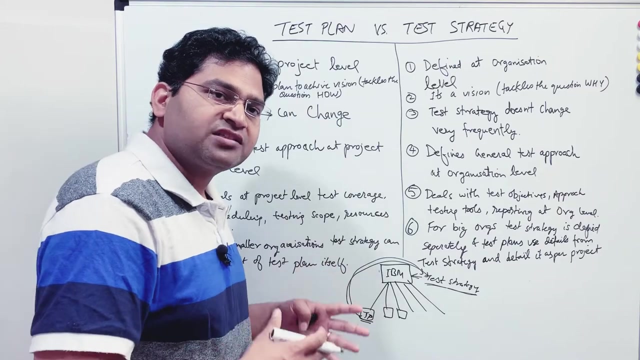 test management tools, multiple defect management processes, and that is the whole point of having a be hundreds of test strategies across those verticals, but then there will be a common test strategy across the org level as well. right, so it is a common understanding or common documentation of the processes, the tools, how the testing will be approached, the artifacts that need. 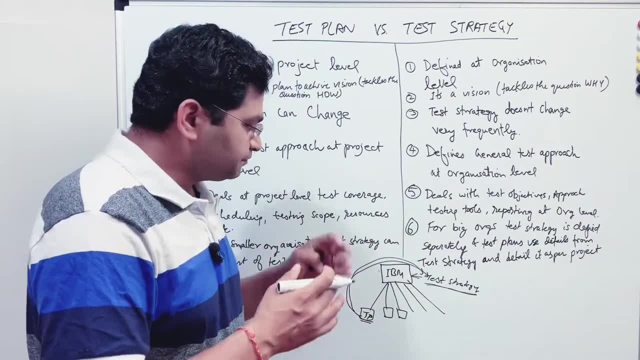 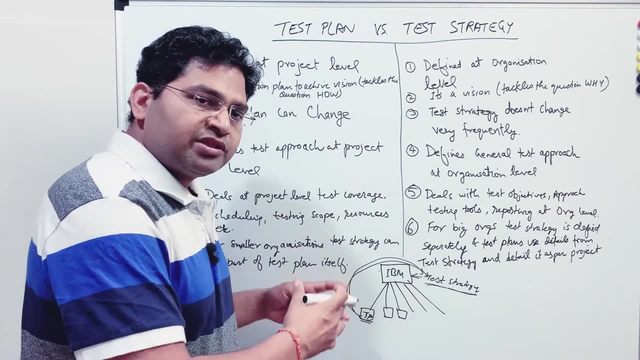 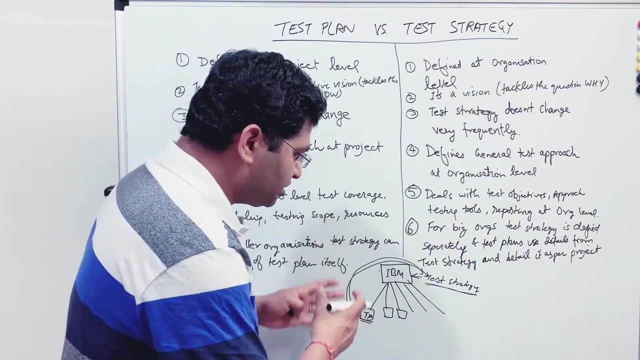 to be generated. that will be defined at the strategy level. when it comes down to the project level, projects refine this strategy as per the project, and that is where the test plan come in picture, and the test plan will have more detail about the project, along with the details from the 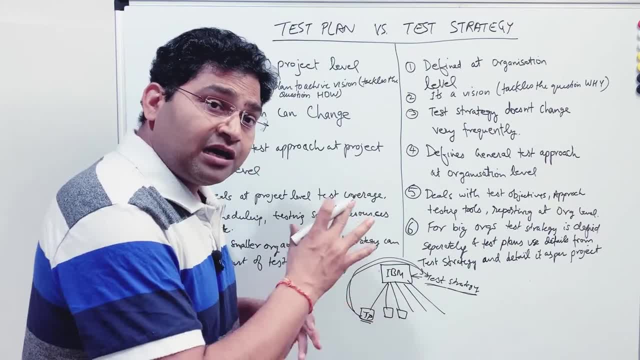 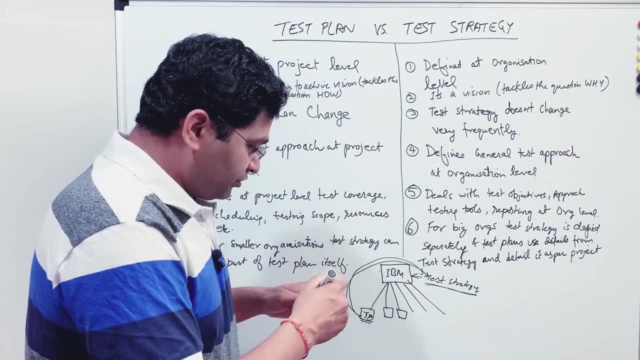 test strategy. so this is basically how the test strategy is written, what is the relevance of test strategy and how the test strategy is related to test plan, right? so this is an example of it. I thought I'll explain this because just reading a bit from a Brian Jones article that I had in the review of a scientific research paper, 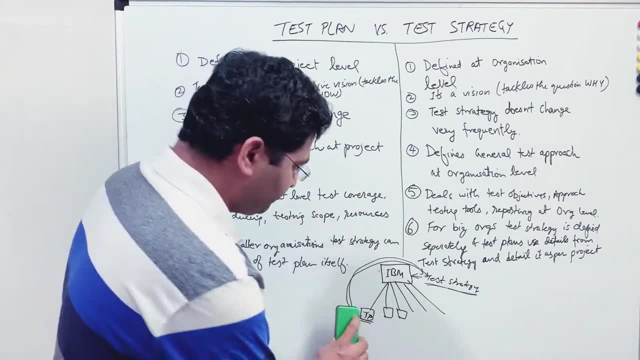 I thought I'll explain this because just reading a bit from a recent research paper I had in the dance, these points won't, you know, help you in the interview. so this is very important to understand. now let's go back to the differences here, or the commonly common. 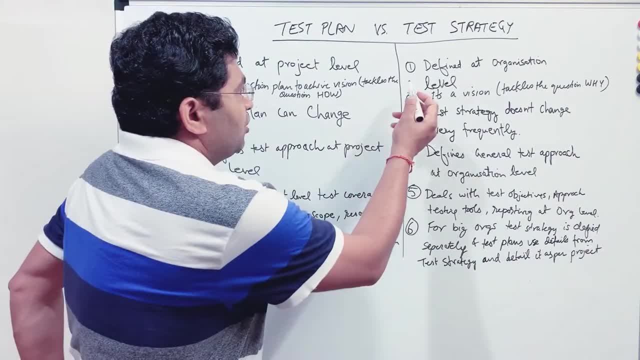 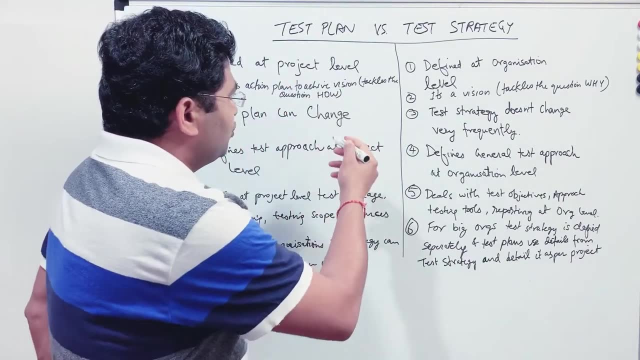 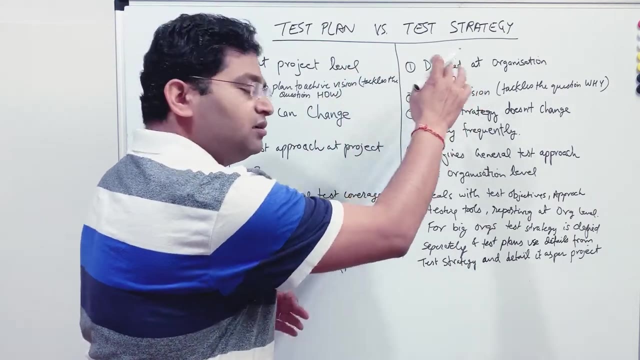 things within test plan and test strategy. so, as I have already explained, test strategy is defined at the organization level. test plan is defined at the project level, which will have more details of the project, specific information, but this test plan will have the information defined at the test. 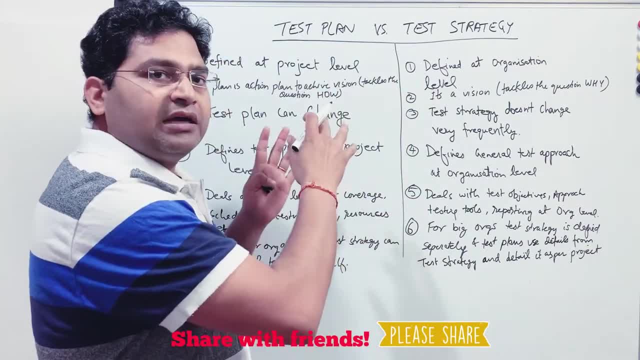 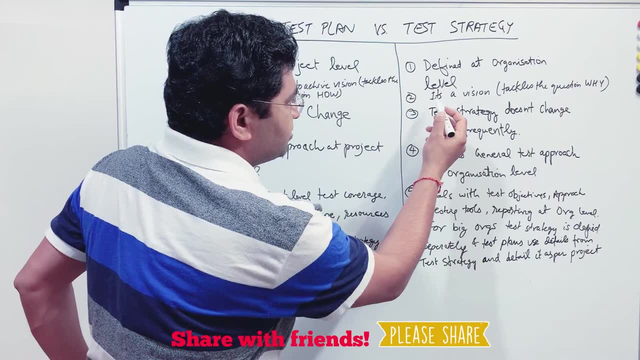 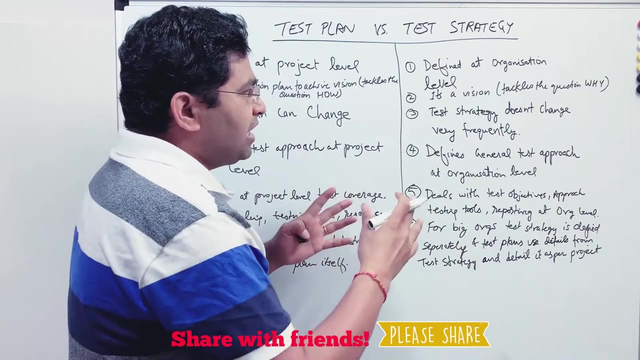 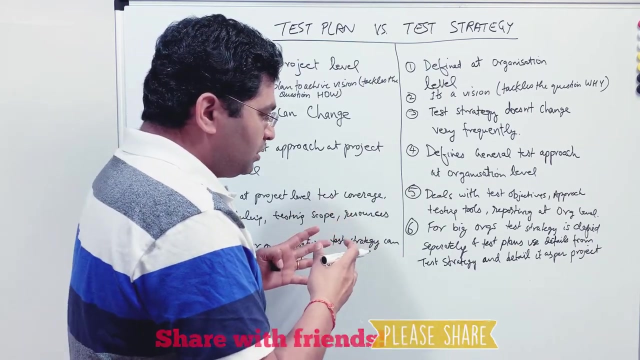 strategy at the org level and elaborate that as per the project. ok, now the second point is basically, the strategy is a vision. so when we talk about the test, strategy tackles the question: why so? why the testing needs to be done in a particular way, why you want to, you know, follow a particular defect management. 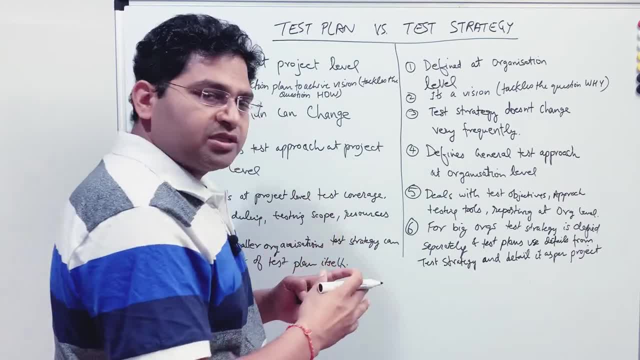 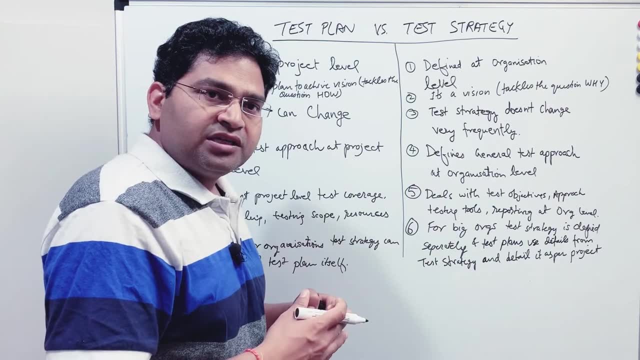 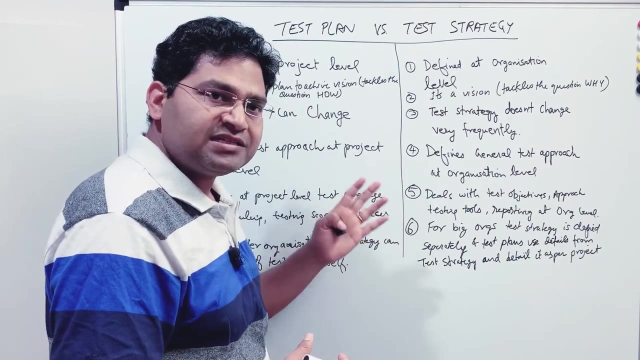 process within the organization so that why question or why part, is basically answered in the test strategy. because maybe your organization is more into medical equipment testing, right? so when you write a test strategy for the medical equipment testing, then that strategy will tackle why you are testing, the why you are performing. 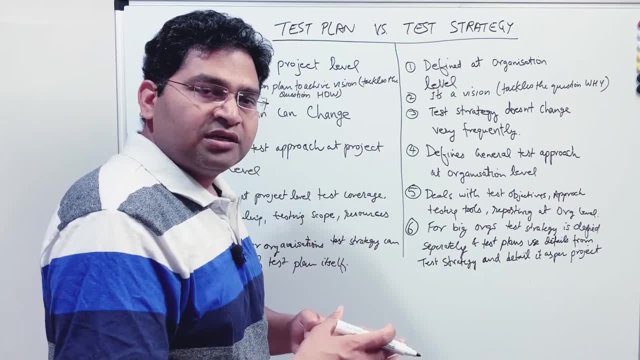 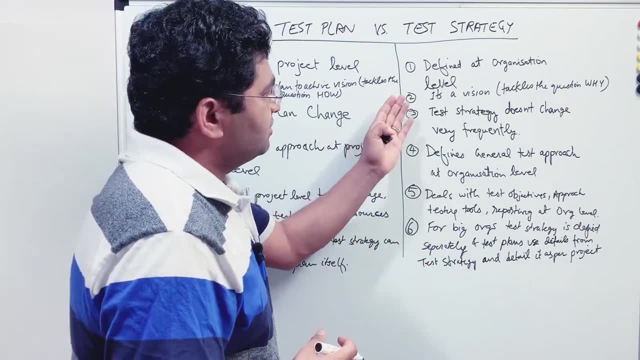 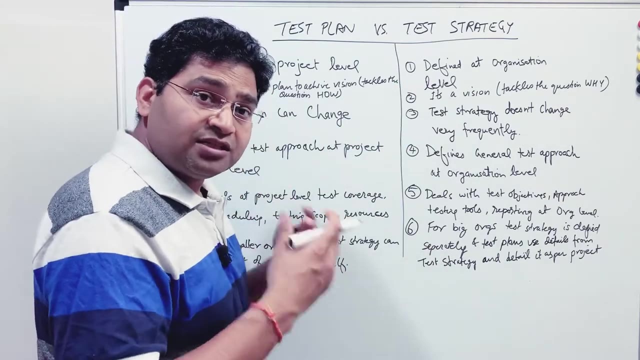 the test process in a particular way for a medical equipment. that is different from the internet applications or e-commerce application, right? so strategy is a vision. it tackles the question why, and the test plan is the plan or the action plan- how you will do the testing for a particular. 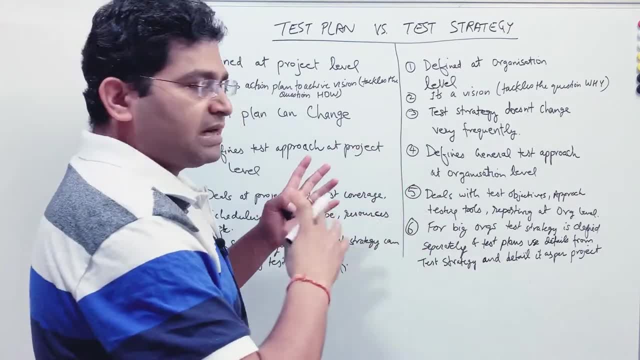 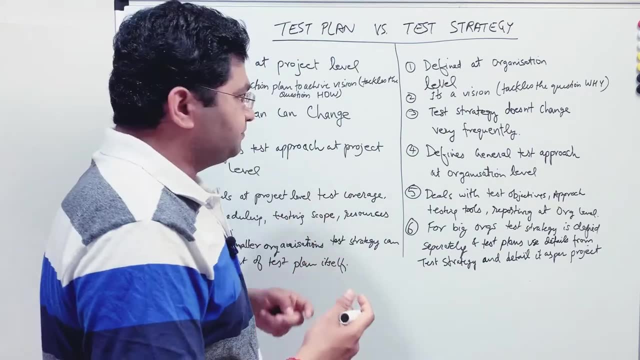 project. so these are the two differences between strategy and plan. so why and how? so how you are going to approach testing is defined into the test plan, then test strategy doesn't change very frequently. so once the test strategy is done, then the test strategy will be done and the test plan 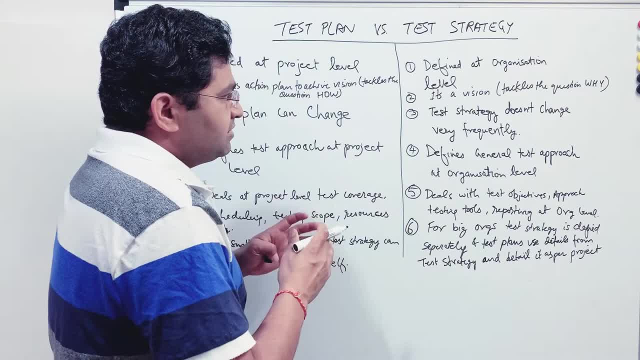 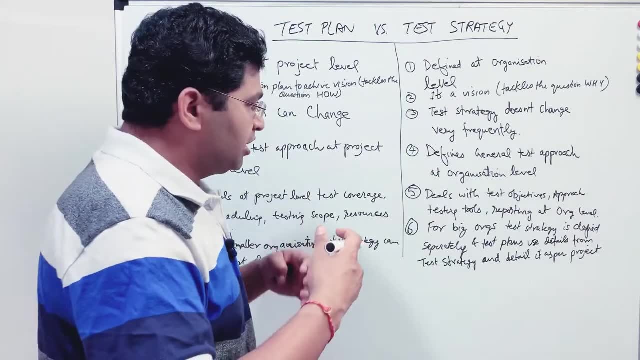 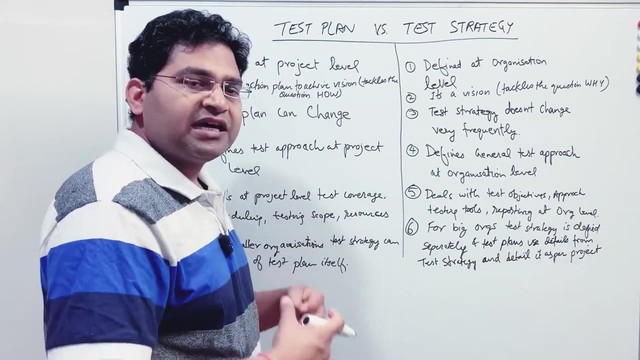 is defined at the organization level. it is not going to change very frequently. however, the test plan can change frequently based on the input. so usually test plan. when you start writing test plan, the first you know you write the draft version. then you refine it as you get more information. 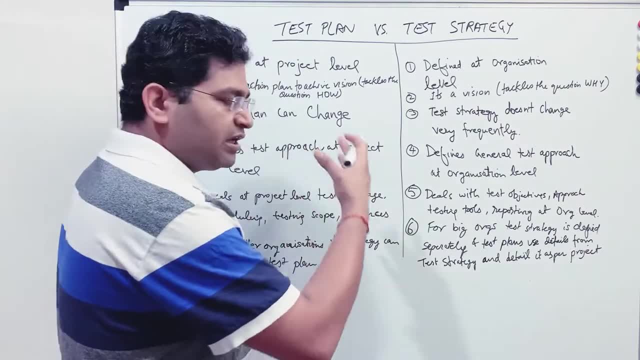 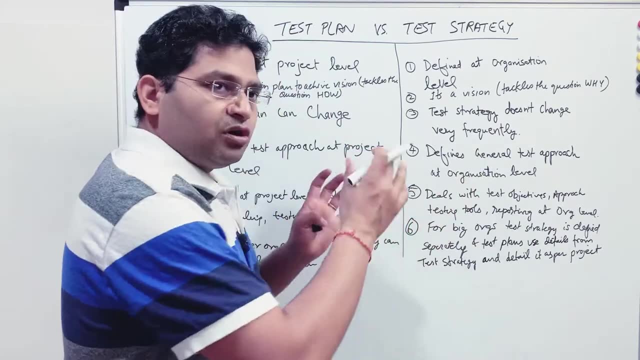 with the from the project you get more detail and you refine and keep changing the plan as per the project progresses. but test strategy is defined at the organ org level and the test strategy is defined at the organization level. and the test strategy is defined at the organization level. 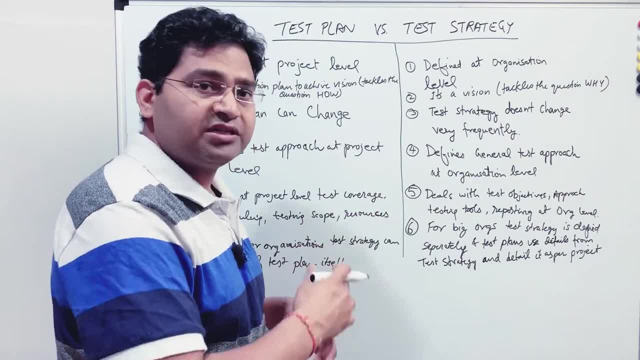 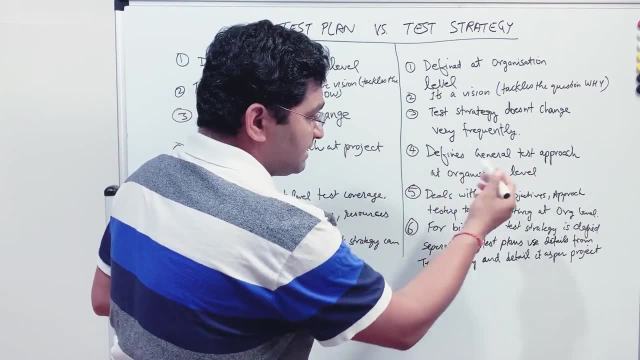 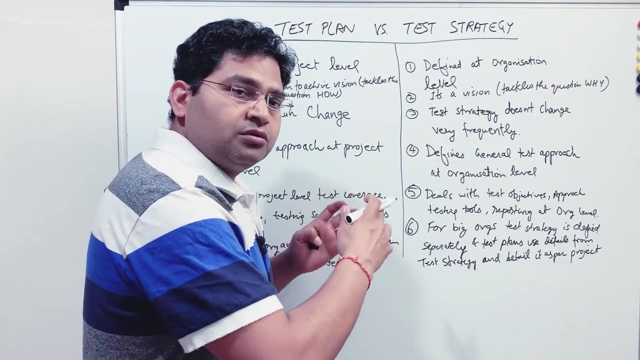 and it doesn't change very frequently. it does change if required, but it doesn't change very frequently. then the fourth point is basically defined test right is defines general test approach at the organization level, which we have already understood with the diagram. so there is a general test approach. what all general you know: tools need to be used, how the defect management. 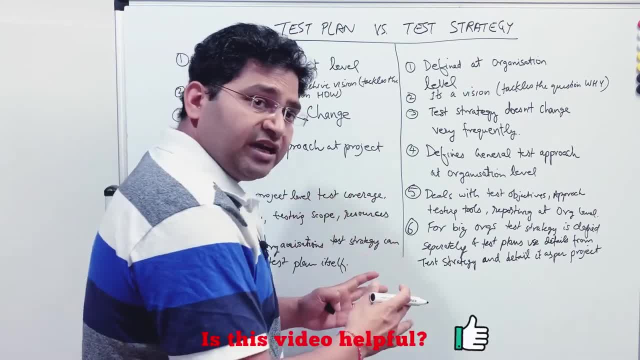 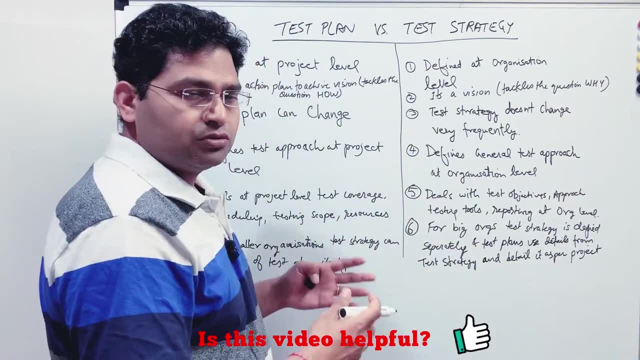 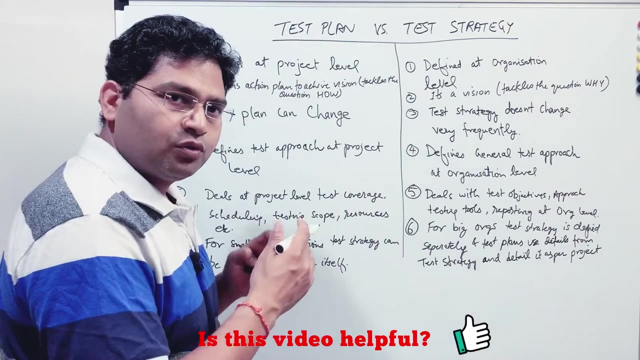 process will be, what artifacts need to be produced once the testing is finished or during the testing. all that generally goes into the test strategy. when we talk about the test plan, it defines the test approach at the project level, so test plan is more of a approach at the 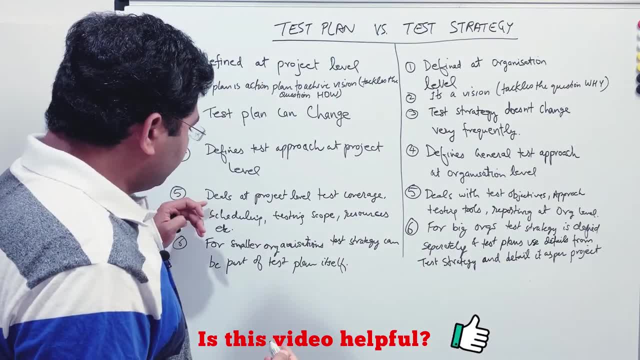 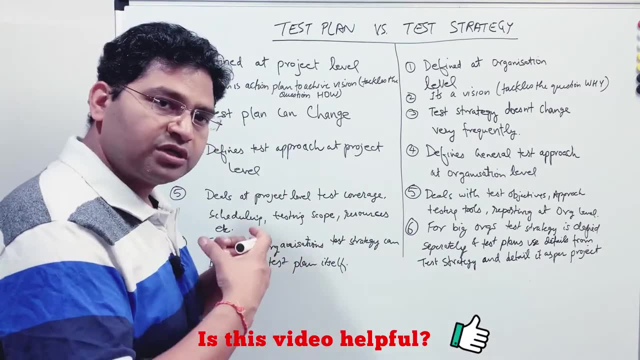 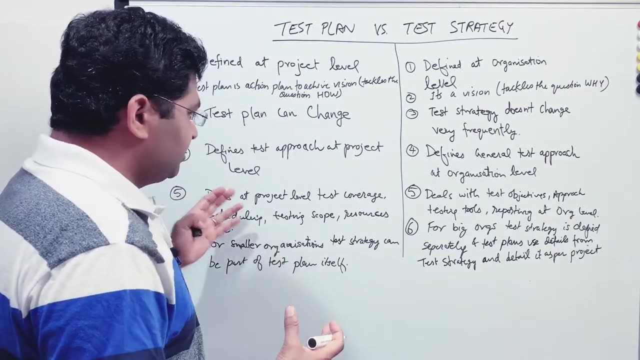 project level, then at the test plan. the next point is it deals with the project level test coverage. the scheduling how the testing will should be scheduled, what resources will be utilized, hardware, software, who will be doing testing, what will be the timeline. all that thing needs to go into the test plan because 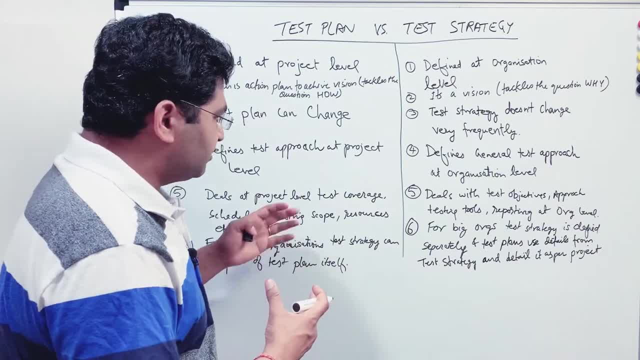 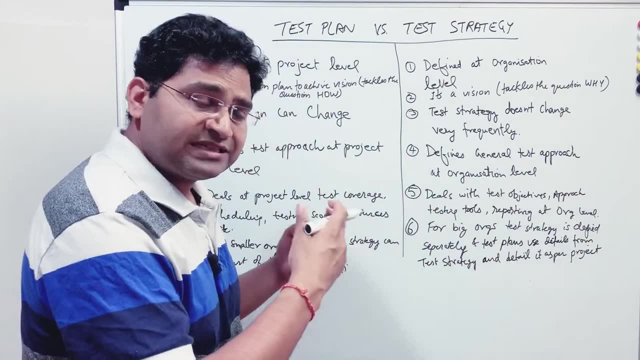 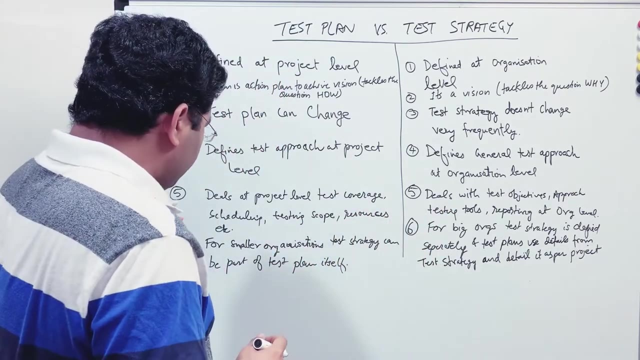 these are the detailed scheduling etc. that goes into the test plan. but when we talk about the test strategy it deals with the test objective, general test approach, what testing tools, reporting etc. artifacts that need to be produced at the organization level. then this, the last point, is basically test plan. if 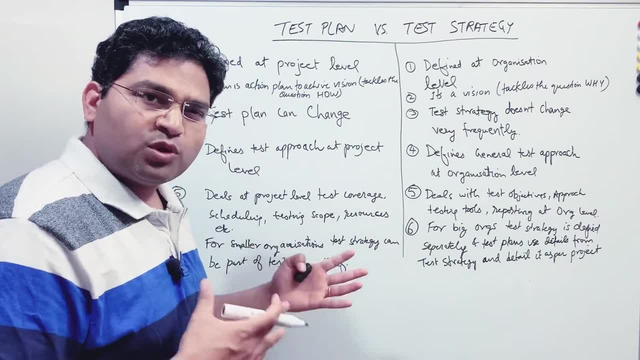 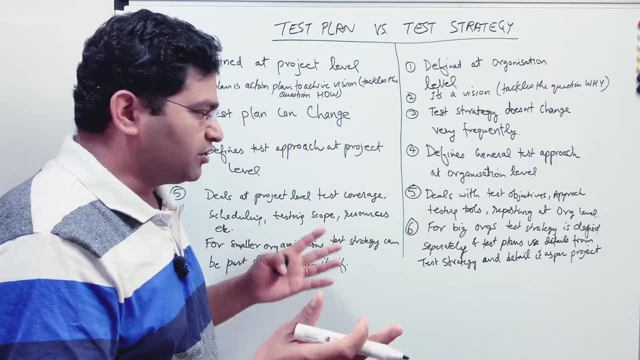 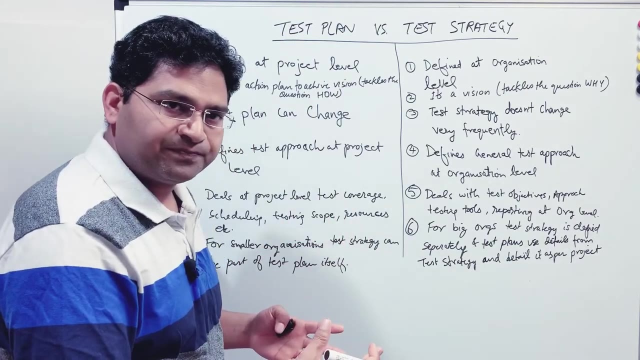 your organization is very small and you have just one or two projects, you don't need to define test strategy and test plan separately for the overall organization. say, for example, your organization is just, you know one or two projects. what you do is within the test plan itself itself. you will have the test strategy right. but in the big